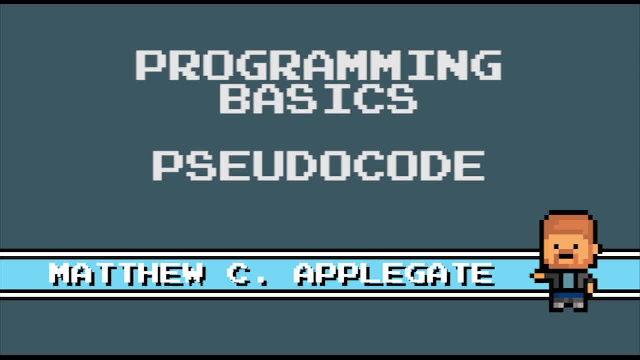 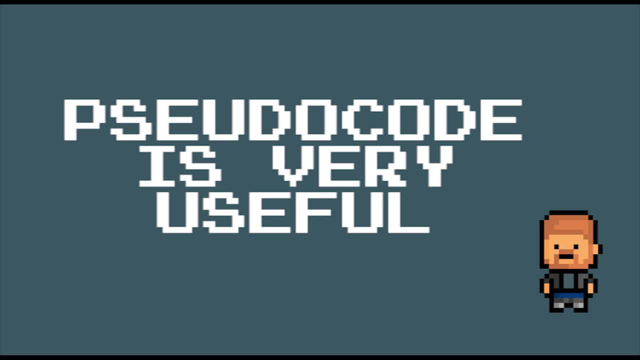 Today we are going to look at pseudocode, So let's look at this in more detail. Okay, here is an example program written in pseudocode. It both does and doesn't look like a computer program. The syntax is similar to most high level computer languages, but at the same time, doesn't have the exact syntax. 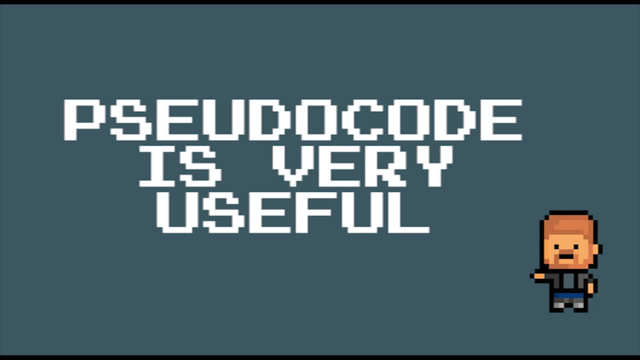 Pseudocode is often referred to as a syntactical representation of a program. Why do people use pseudocode? Well, it has two very useful uses. Firstly, it can be used to help non-programmers understand what is happening in a program. 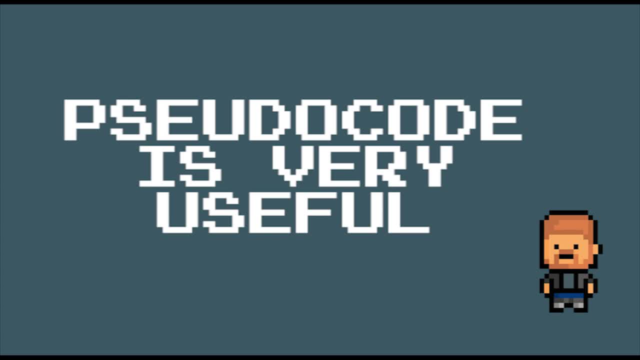 The second use for pseudocode is for when programmers are trying to debug and solve simple problems. This is where you can learn more about pseudocode. You can see a lot of examples in the clip. Now let's go over them in the description. 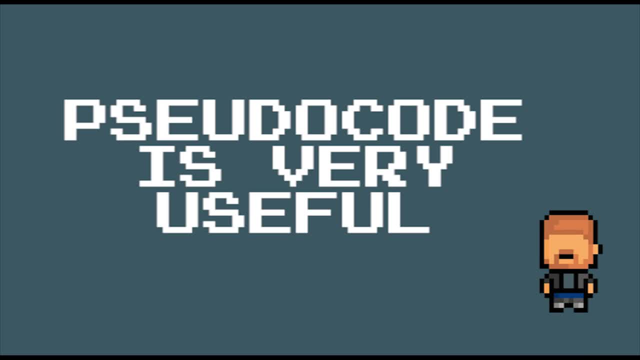 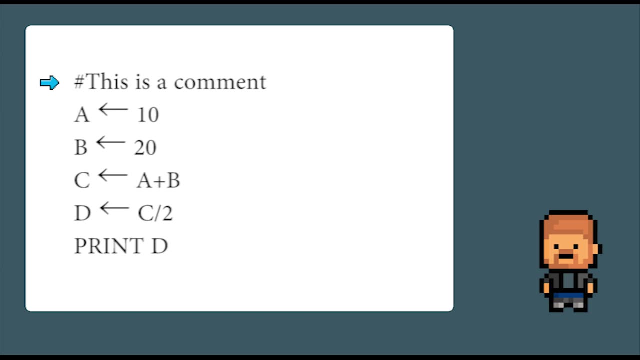 a logic error in a computer program. as it is closer to spoken language, it often helps programmers find where the program is going wrong. let's look at our first program in pseudocode. okay, the first line is pretty straightforward: it is a comment. a comment is ignored by the program and is used for us humans to 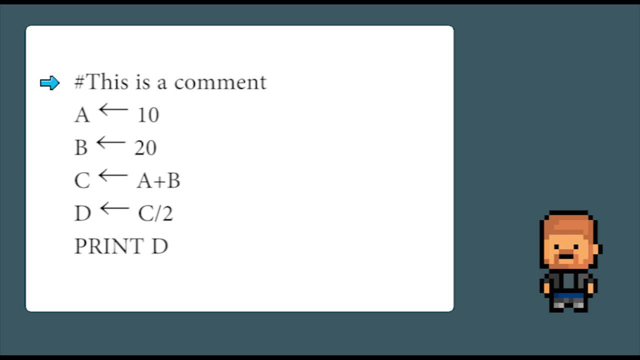 read. it helps us remember what something does and if you are part of a team of programmers, it can help explain what it does to another programmer. the second line, the a variable is assigned the value of 10. this arrow means assignment. it is similar to a single equal symbol, in this case a equals 10. the same thing. 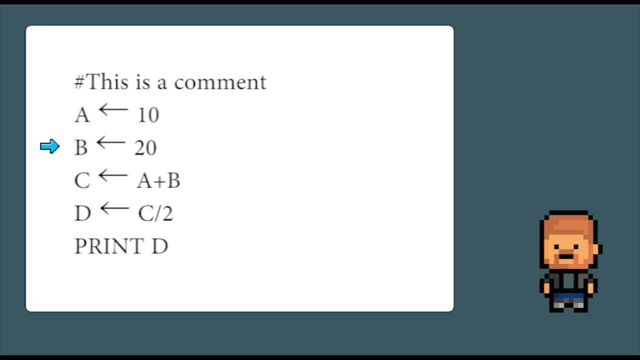 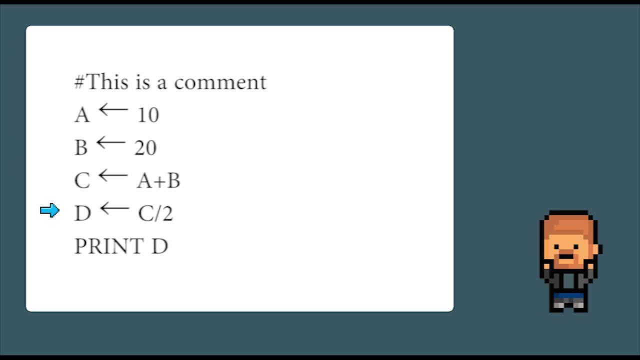 equal to 30, aligned 5. D is being assigned C. divided by 2, this effectively half 30 to 15. so D is now being assigned 15 and finally, print D. this is an output command. it takes something from the computer program and shares it with the 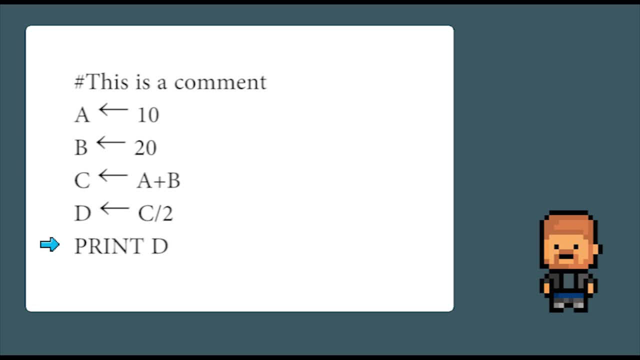 real world. it outputs the value of D to the screen, which in this case is 15. so there you go. you can have comments, variables and outputs in pseudocode. but that is just the beginning. in fact, most things can be achieved in pseudocode. let's look at another short program.